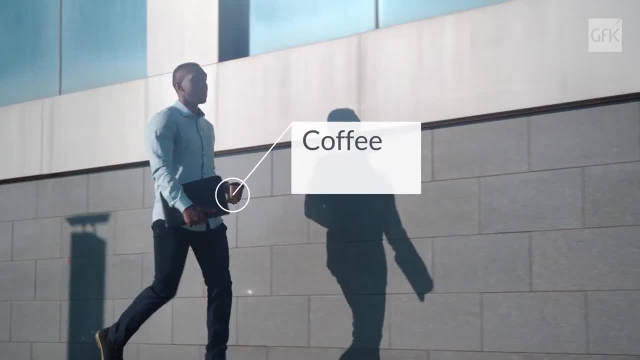 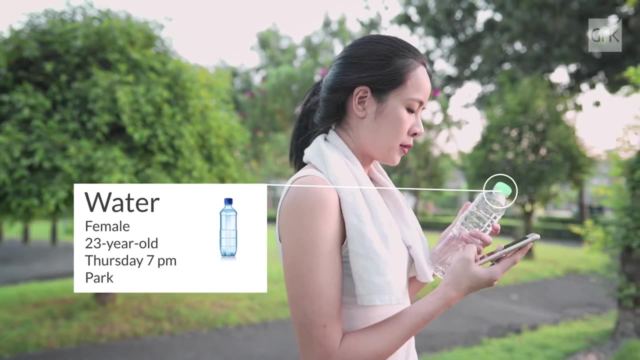 recording all meals and beverages that are bought outside the home for consumption. This can be, for example, a water from the gym or bought at the supermarket, just as much as a visit to the canteen at lunchtime or a cappuccino from a café. 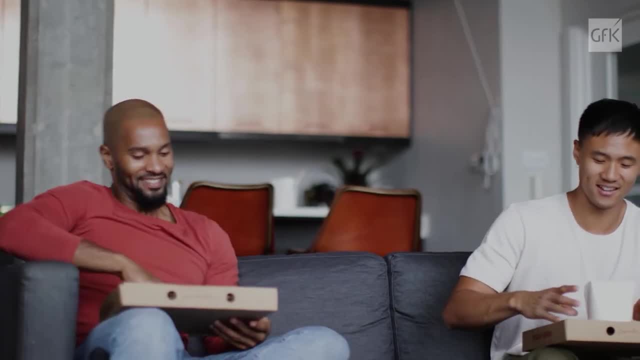 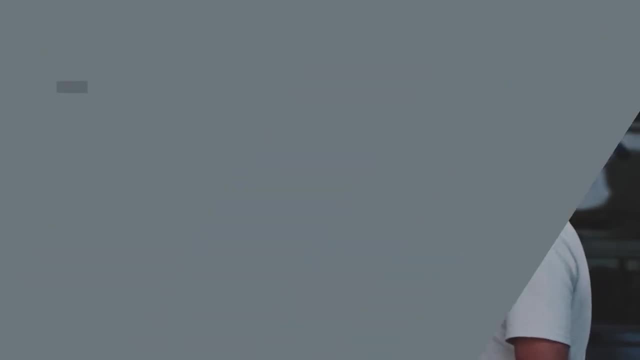 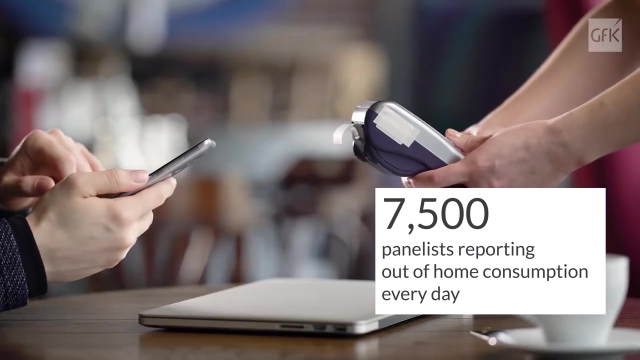 The same applies to home-delivered or takeaway meals from delivery services, snack bars or restaurants, or cocktails with friends at a bar. GfK Out-of-Home Panel captures all these meal and beverage occurrences in various out-of-home market channels. Our motivated 7,500 panellists report their out-of-home consumption on our platform every day. 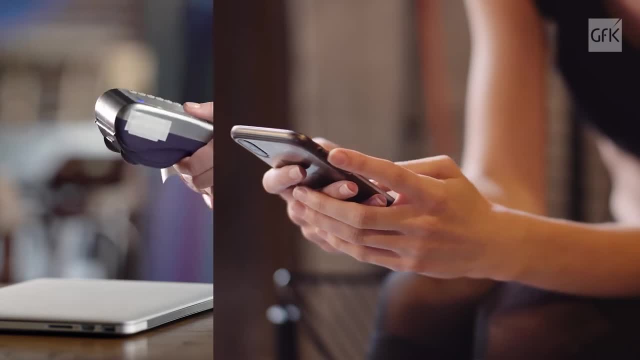 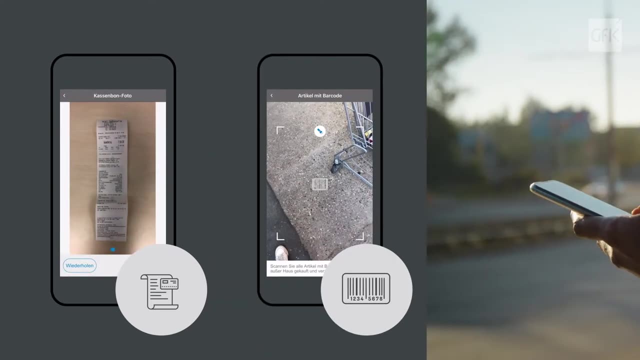 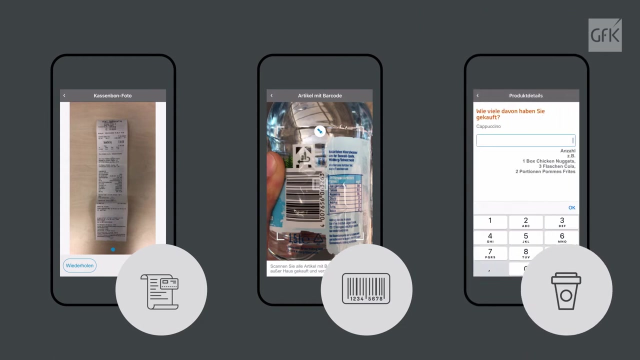 using innovative technology that enables recording in just a few seconds by photographing the receipt, scanning the product's barcode or entering the purchase with a few clicks on the screen. The data collected by panellists is carefully reviewed and aggregated by our industry experts at GfK. 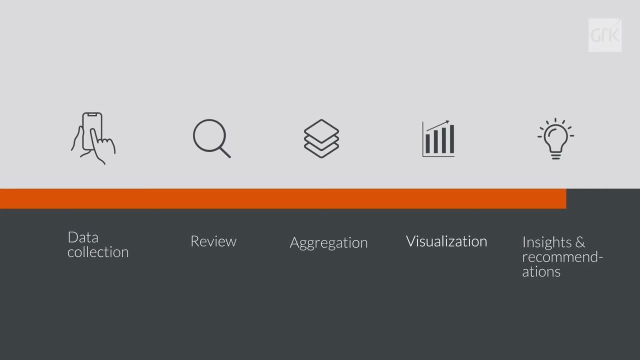 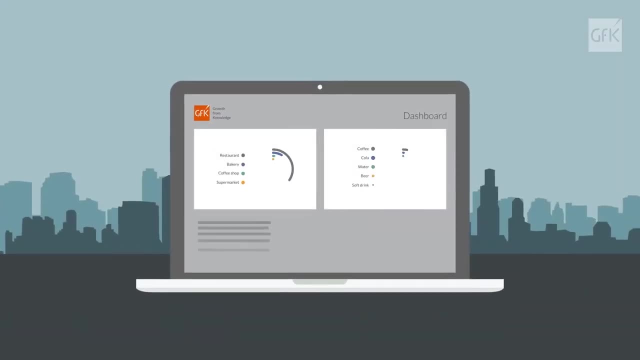 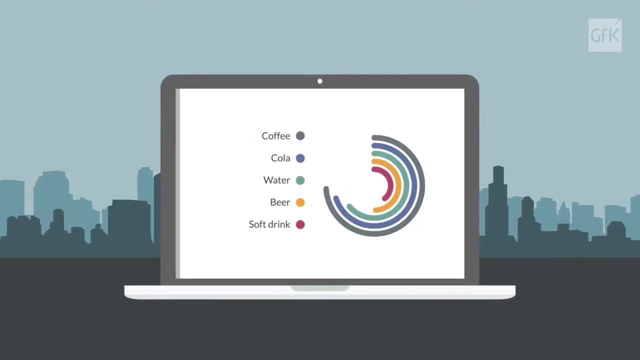 using next-level technology to give you modern visualisations and fact-based insights that can help you make the right business decisions. We can identify all relevant out-of-home market channels for your brand based on real purchase data, and break this down even further according to the products or dishes. 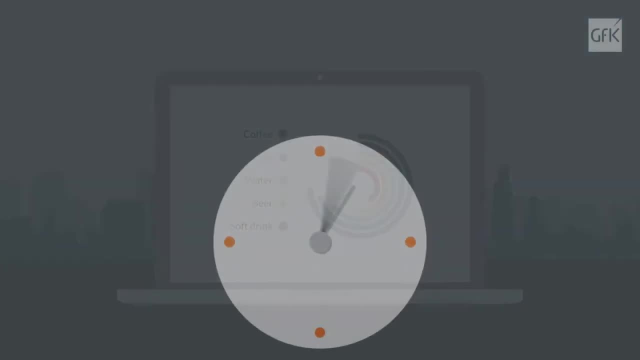 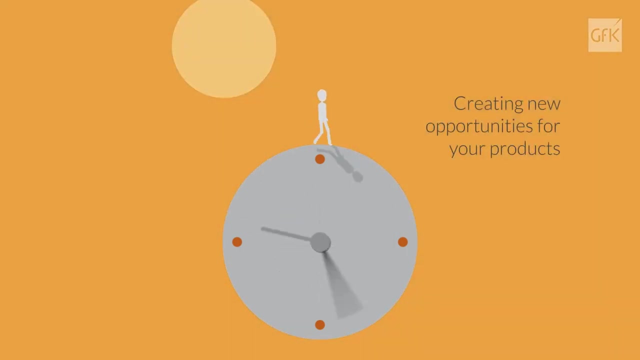 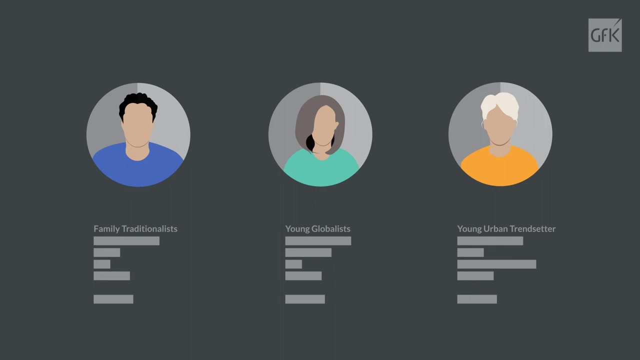 that are most important to your target customers, so you can understand the consumption habits of your consumers throughout the day and create new opportunities for your products. With our GfK Out-of-Home Panel, you get to know your target group even better and can address them more effectively. 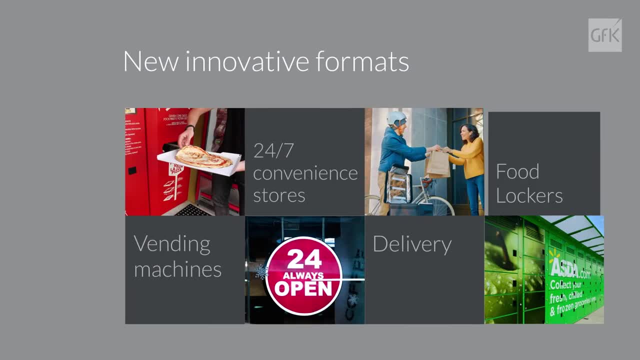 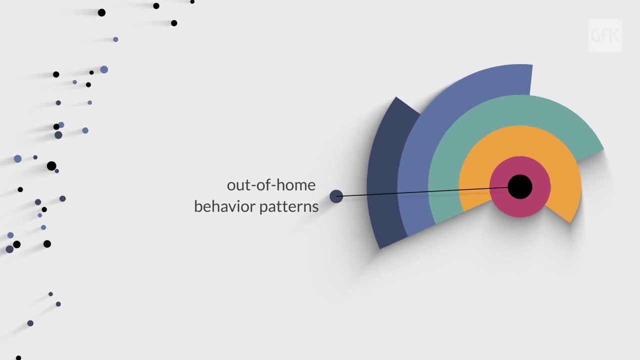 avoiding costly advertising efforts leading nowhere. Our insights help you to drive innovation. With GfK Out-of-Home Panel, you will find the unique drivers for your success in the out-of-home market. understand and influence your target consumers' behaviour patterns. 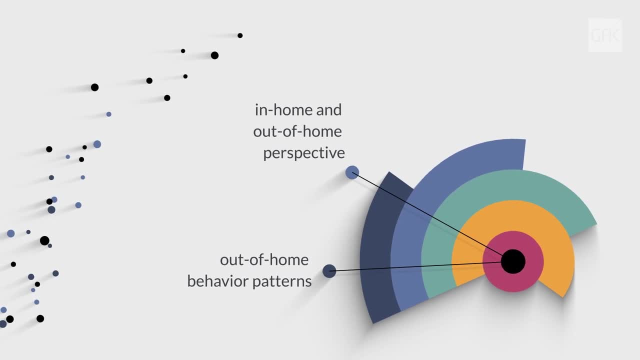 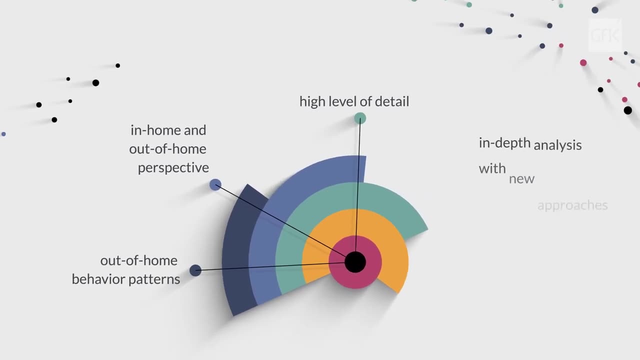 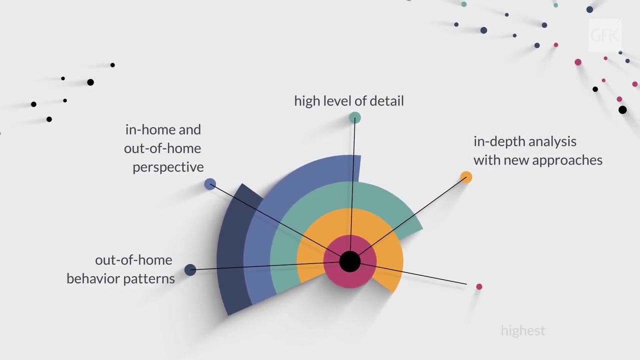 bring together the in-home and out-of-home perspectives for a holistic view of your company's potential. benefit from the high level of detail from our data and in-depth analysis and new approaches made possible by long-term consumption histories. You can always rely on the highest data quality.